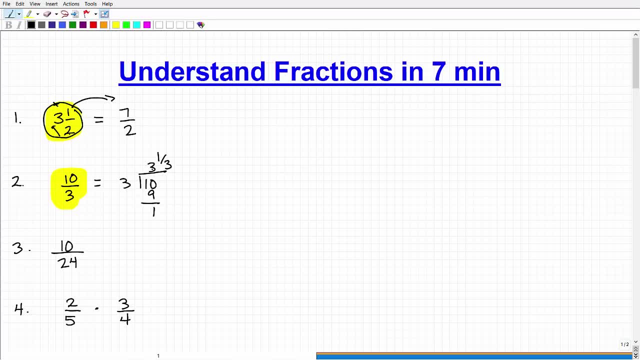 This is is 3 is. We're going to write it just like this. so that's 3 and 1 third. so 10 thirds, Okay, is equal to 3 and 1 third. so just basic fraction terminology. This is an improper fraction Because the numerator matter of fact. 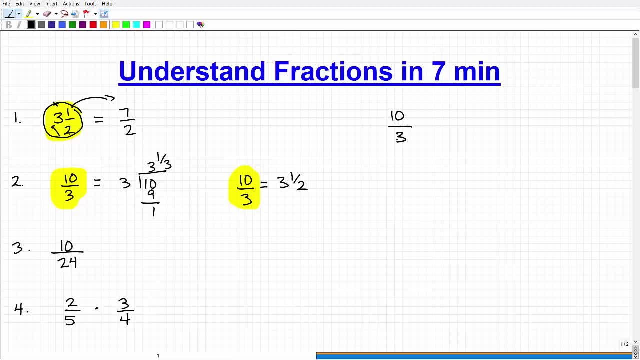 I should just kind of break this up here: 10 over 3. when we're dealing with fractions, The top number is the numerator, the bottom number is the denominator. Okay, so anytime the numerator number is bigger than denominator number, we call that an improper fraction. Now I talked about mixed numbers. Okay, so I can write this as: 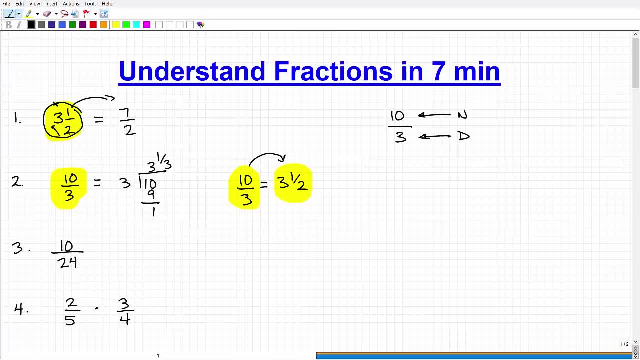 3 and 1 half, so this is a mixed number. This is an improper fraction, And a proper fraction is where the numerator is less than the denominator, So something like 1 half. Okay, so the denominator down here is bigger than the numerator, So this is a proper fraction. 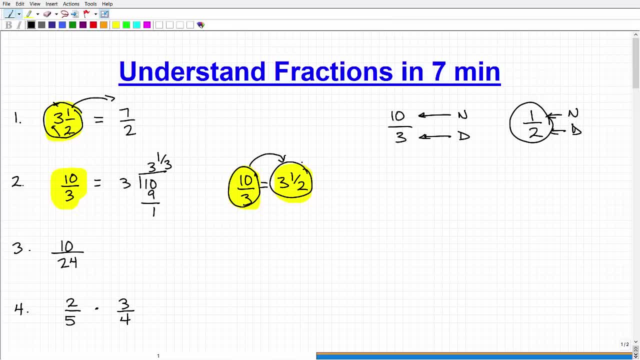 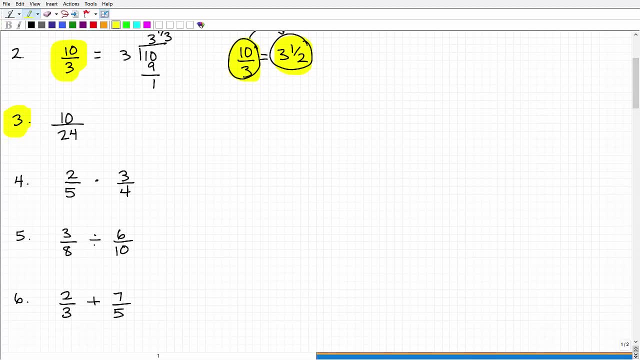 Improper fraction and mixed numbers, So you need to kind of be able to go back and forth between the two. Okay, so we're on the number 3 And let's see here. so in this one I wanted to talk about very quickly the idea of reducing or 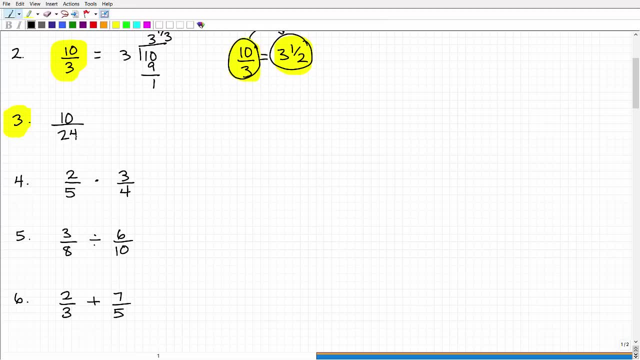 Simplifying your fraction. So here I have 10 over 24. when you're dealing with fractions, You always want to reduce them or write them in their simplest form, So the idea here is to think of a number that goes into both 10 and 24. 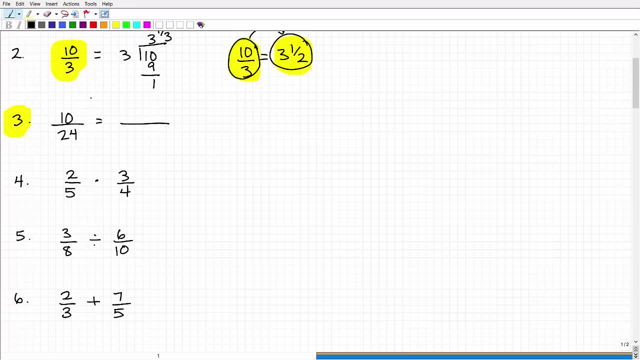 So you might have thought to yourself: Well, it's 2.. Okay, and that's good. So 2 goes into 10- how many times? 5 times. and 2 goes into 24, 12 times. Okay, so this fraction 10, 24, 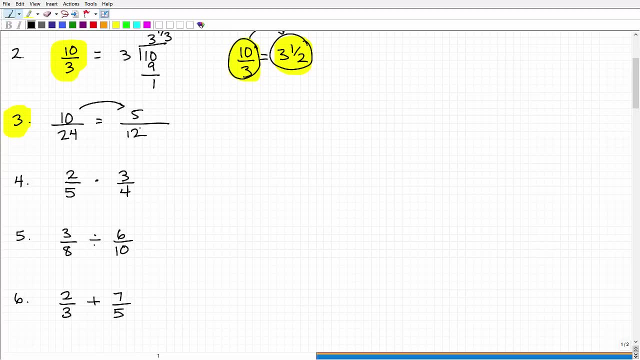 is Equivalent to the simpler fraction 5, 12. now another way you can think about reducing or simplifying fractions. Let me go and write this over here: 10, 24, s is to look at the factors of these numbers. In other words, 10 is the same thing as 2 times 5, and 24 is the same thing as 2. 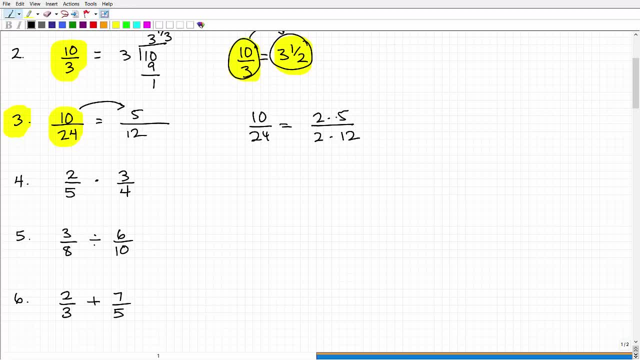 Times 12.. So anytime you have the- and these are called factors again. okay, now where This 10 can be written as a Product of these numbers, These are the factors of this number here. but anytime you have the same factor in Both the numerator and denominator, we could do something called cross cancel, essentially just get rid of them, and then whatever is left is: 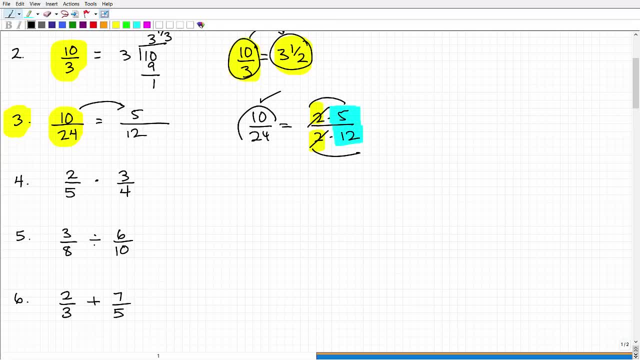 The answer: okay. this is more the simplified fraction. So 10 24th is Equivalent to the fraction 5- 12.. Okay, so We talked about the basic part so far: fractions, numerator, denominator, Proper fraction, improper fraction, mixed number, and now simplifying. so remember, when you're dealing with fractions, you always want to work. 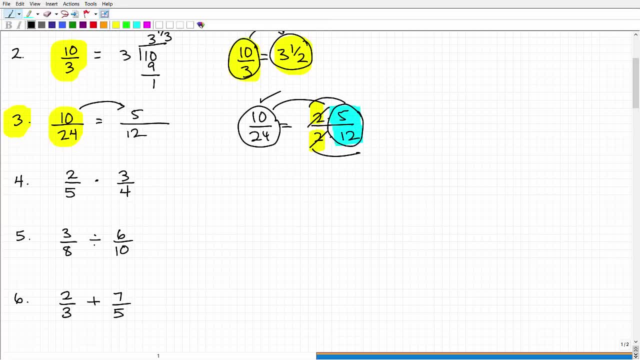 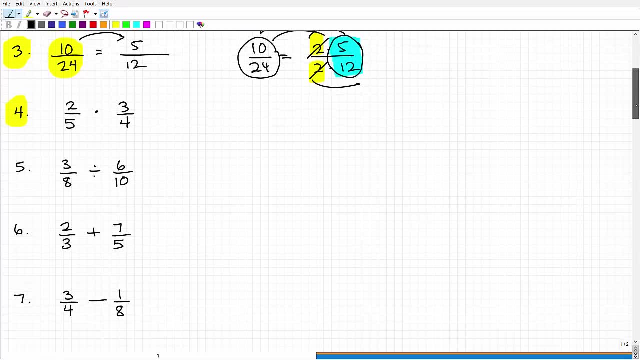 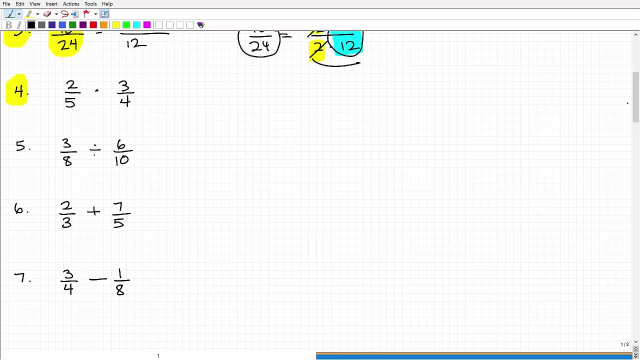 With fractions in our simplest forms. or your final answer. you want to reduce? Okay, All right, let's move on to number four. Okay, so hopefully I can get this done in seven minutes. I may go over a little bit, but Just think you'll. you'll understand fractions here, crash course, All right, so now we have two fractions here. 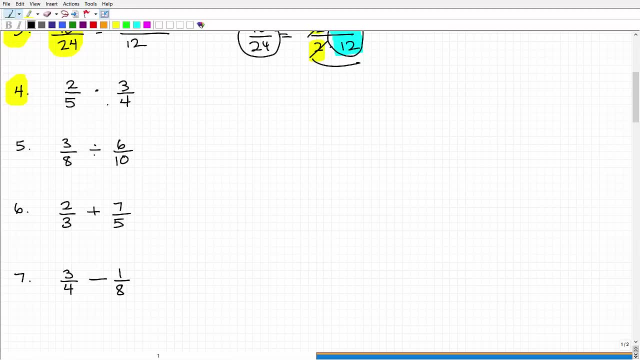 Doesn't make a difference. if they're improper, proper, Okay. But the idea is we want to multiply them. So I have one fraction and I want to multiply it by another fraction. This is very easy, Okay. all you need to do is simply multiply The respective numerators and denominators. so 2 times 3 is 6. 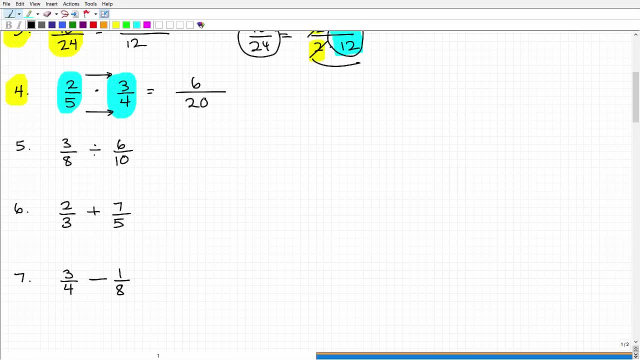 5 times 4 is 20. okay, and then here This is a valid, correct answer. However, you always want to simplify Your answers. reduce it. Okay. this was kind of brings us back to the previous problem. So you can think of 6 as what? 2 times 3, as I just wrote this, in 20. 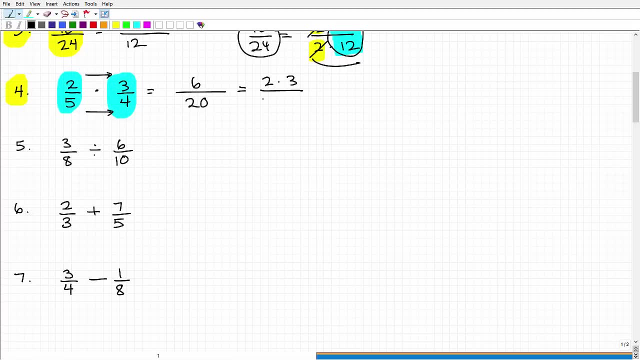 I can think of- well, I think it was 5 times 4, but I can also think of as 2 times 10, because I'm looking to create kind of common factors, so I could cross, cancel and I'm left with the Fraction 3 tenths. Okay, so 3 tenths is the. 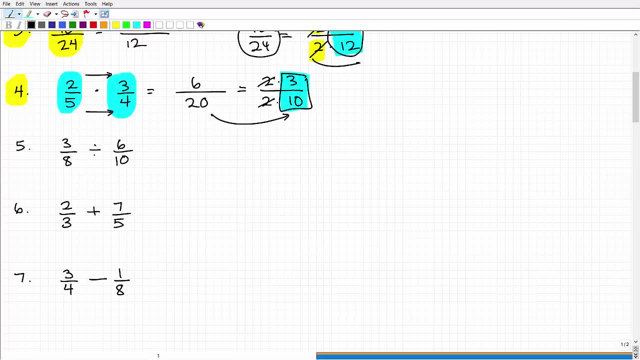 Simplified version of 6- 20th. mathematically they're equivalent, Okay, but you always want to leave your final answers Fully reduced or simplified. Okay, so we've got multiplication down. Let's talk about division. So division is actually quite easy as well. 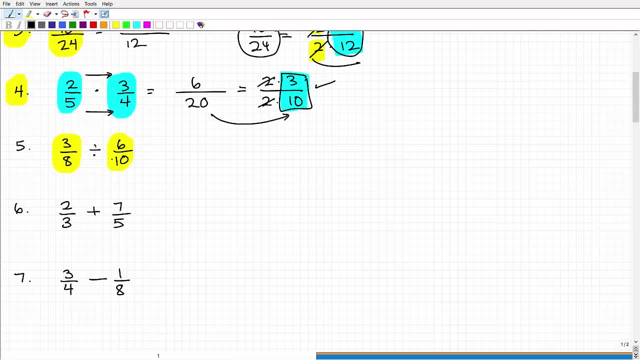 What we do with fractions is we don't actually divide fractions. we're going to turn this problem into a multiplication problem and because the previous Problem here I showed you how to multiply, So we already know how to do that- I'm going to ship. we're going to turn this into a multiplication problem and then we're going to do what we did in problem before. 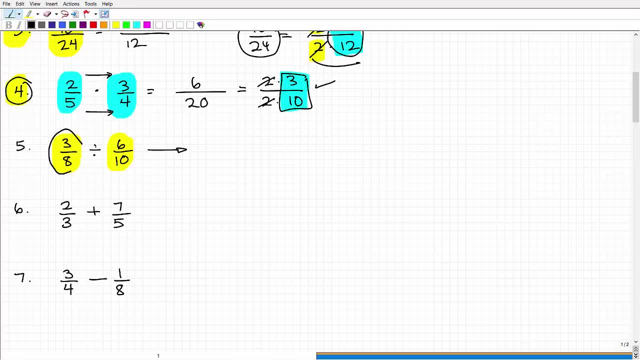 So what we do there- it's very easy- is where we write the first fraction again, So that's 3 eighths. Now we're going to change the division sign here into multiplication. Now here's the deal in order to change this from division to multiplication. 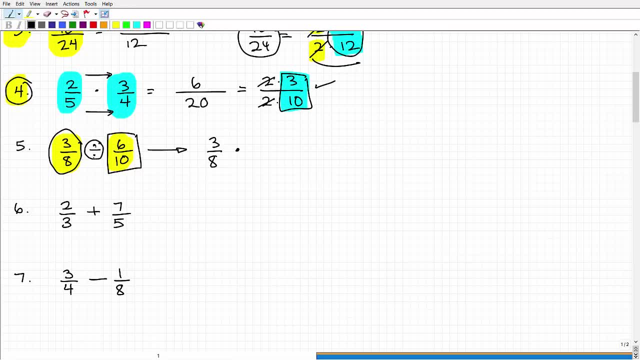 You have to take this fraction to the right of the symbol, the division symbol, And flip it upside down. It's called the reciprocal or inverse. just flip it upside down. So that's going to be 10 over 6. Okay, so now I have a multiplication problems. I'm going to do what I did in prom before. Okay, I'm simply going to. 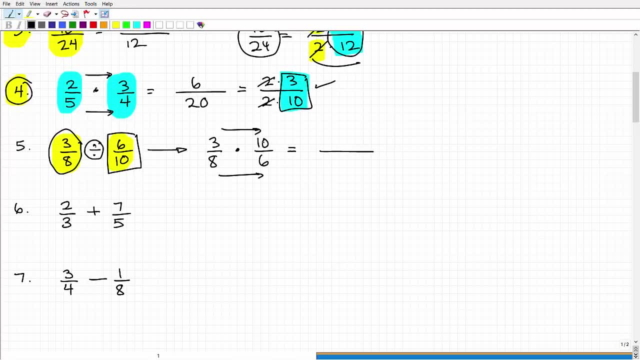 multiply the respective numerators and denominators. so 3 times 10 is 30 and 6 times 8, of 8 times 6,- excuse me- is 48, and then I would go ahead and simplify. I'm actually going to skip that right now because I want to try to see if I can finish this video up in a pretty 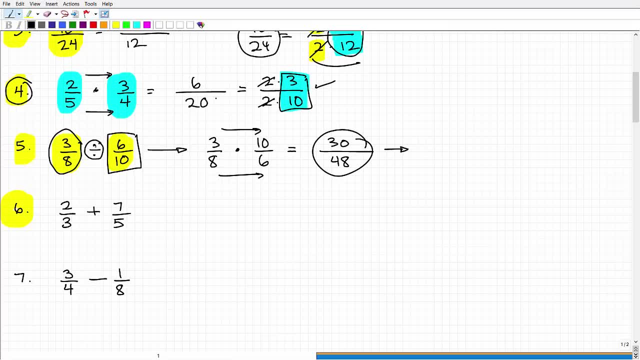 Timely manner. However, we would want to simplify, as I showed you in problems 3 & 4. Okay, but technically speaking, all right. this is a correct answer. now Let's kind of stop and pause, if you think about the operations that we do with numbers. 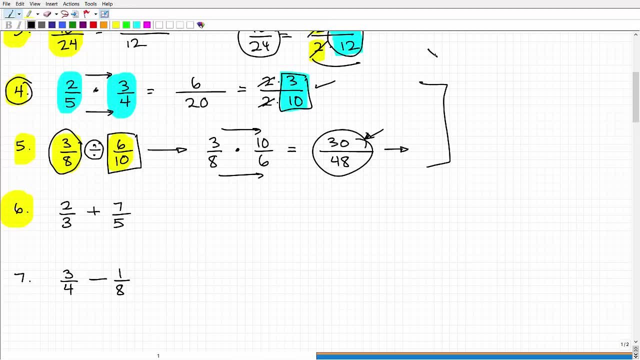 You can. fractions are nothing more than numbers. We multiply, we divide, we add And we subtract. so, as I showed you, with fractions, multiplication or division are effectively the same Step. we have to take an extra step with the division, but we end up just multiplying. The same thing is going to be true with addition and subtraction. 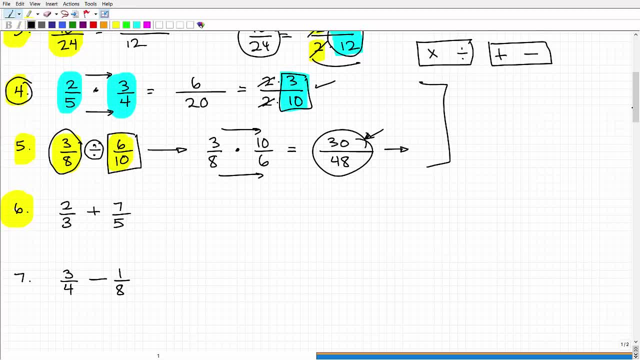 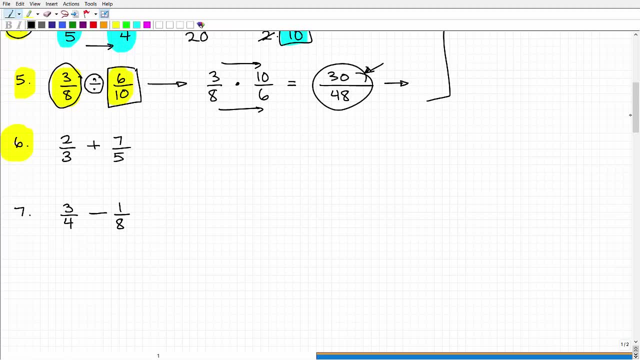 Effectively. you're going to do the same things now For the purposes of this video, because I'm gonna direct this video towards somebody who's, like, maybe totally forgot fractions or really struggling, but I'm going to teach you, you a way to add and subtract fractions, um, that we're going to bypass what they kind of teach you. 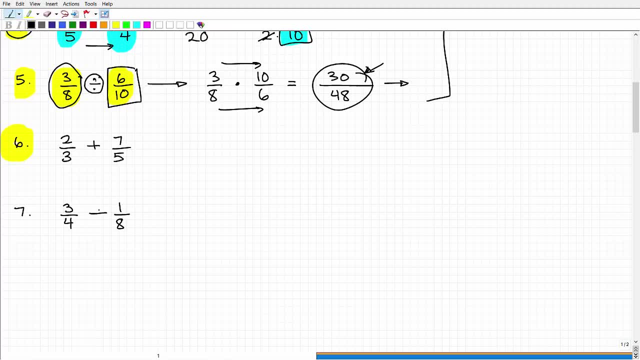 in school as far as the lowest common denominator and all that kind of good stuff. so i'm going to give you a shortcut method. the idea here is that i'm just giving you a procedure to use that you'll get these problems right every time. okay, so let's talk about addition and subtraction. procedure is: 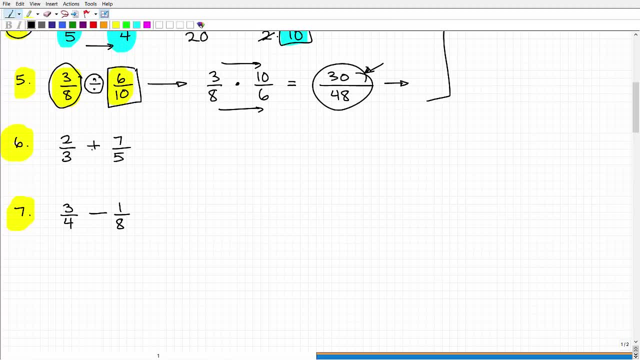 the same. okay, no matter what, uh, whether you're dealing with adding or subtracting. so here goes. it's called the bowtie method, so the way it works is this: you start with this number down here. okay, so it's the fraction to the right. okay, it actually doesn't have to be in this particular. 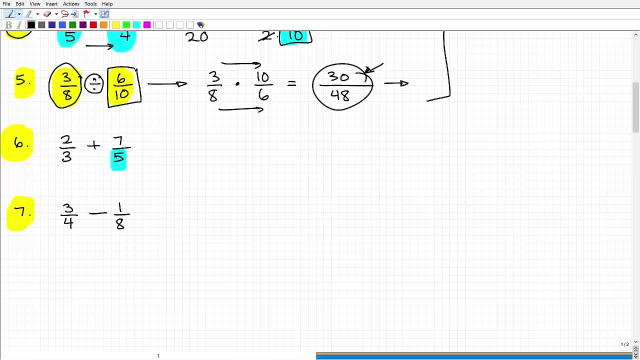 order, but this is the way i do it. i would suggest you just do it my way and just remember the. this procedure is three steps and you'll be done. so it's going to be this number times this number, so let's go ahead and write that here. so five times two is what ten? we'll write that there. 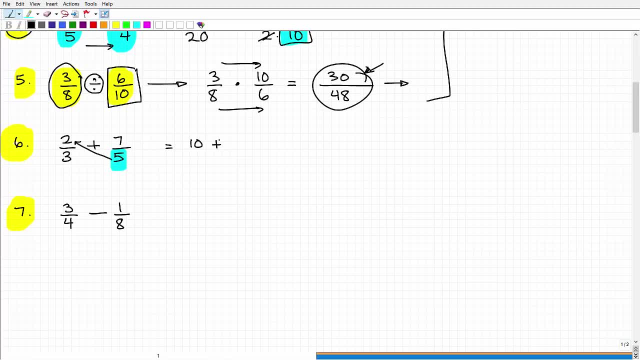 this is an addition problem, so i'm going to write a plus, then you're going to take this number and we're going to multiply across this way. okay, in a diagonal fashion. so three times seven is 21. okay, this is our numerator, so we're going. 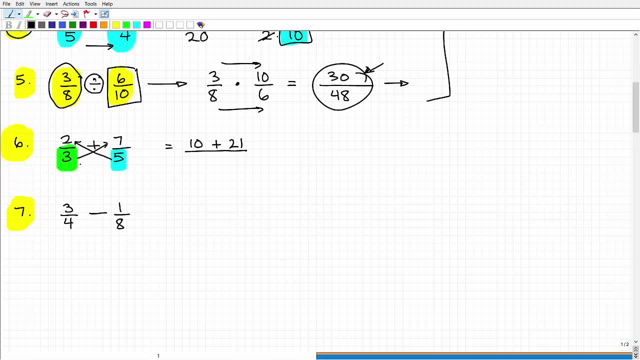 to draw a little fraction bar. now, to get to our denominator, we just simply multiply the bottom numbers, okay, so three times five is 15, and we just simplify this. 10 times 21 is 31 over 15, and you're done. that is it. so this is a great method, because when you're dealing with algebra, 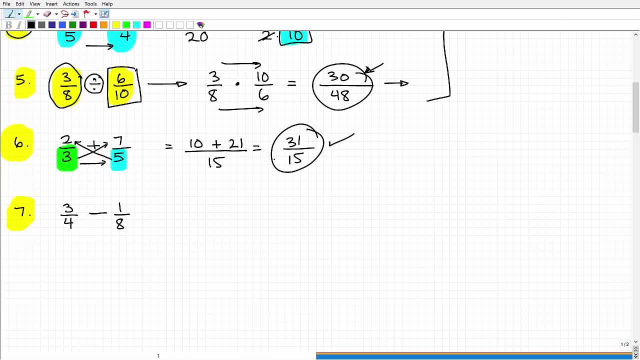 by the way, let me just say one other thing here. you would want to simplify this uh answer. so if you got an answer, let's say 30 over 48 or something you want to simplify uh the answer. the disadvantage for using this method for all problems is that sometimes you won't be you'll. 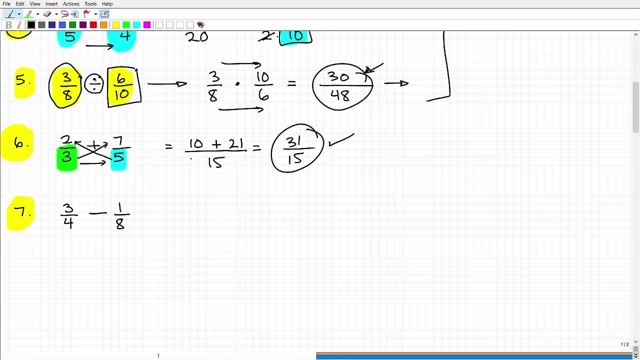 you'll get a fraction that doesn't have the lowest common denominator, Um. so technically you you still need to understand that if you're in a algebra course or whatnot. but but doing it, but adding fractions, this way you'll get them right. 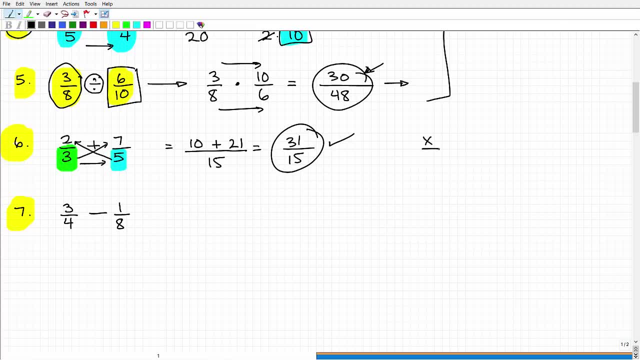 every single time. And by the way it says: take a look at a quick algebra problem. Let's say, I have something like this: Um, so you may not understand this completely, but if I wanted to add these fractions, I could go X times X. 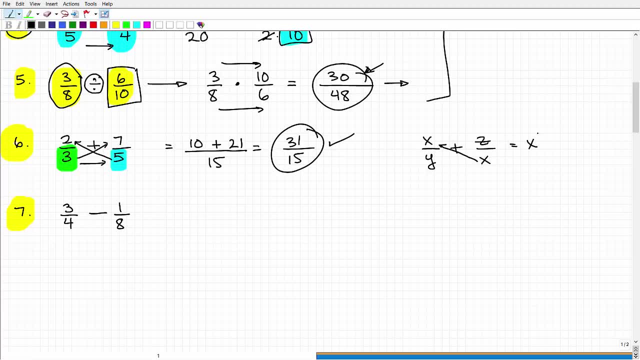 I'm following the same step. X times X happens to be X squared. Okay, Y times Z. Sorry, this is an addition problem, So it's going to be plus Y times Z. is Y Z over Y times X, And that's it. 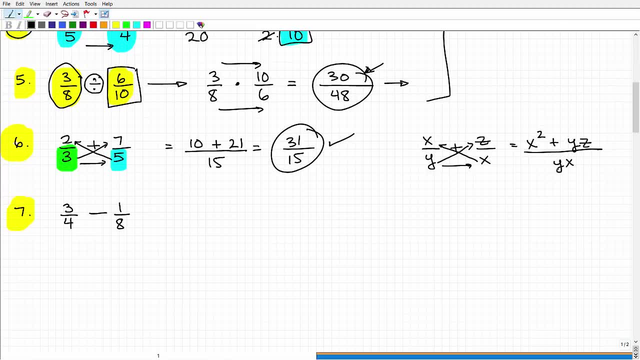 This is a great method. I refer to it as a bow tie method. So, um, you definitely want to learn this, or keep this in your kind of like back pocket, Okay, So if you forget anything about fractions, you can always do this for addition and subtraction. 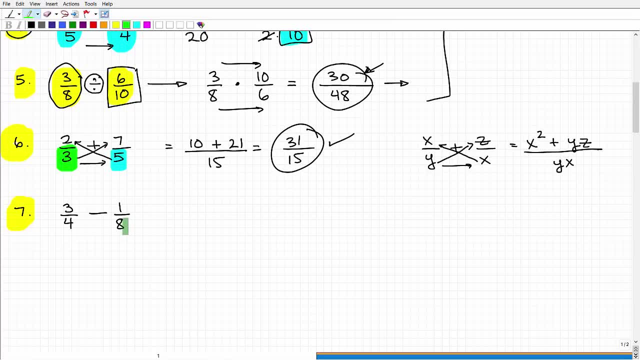 Okay, Let's do this last problem. here We're using the exact same method, Starting with this bottom number. We're going to go this way Eight times three is what? Twenty four Now, because this is a subtraction problem we need. we need to use a subtraction operator. 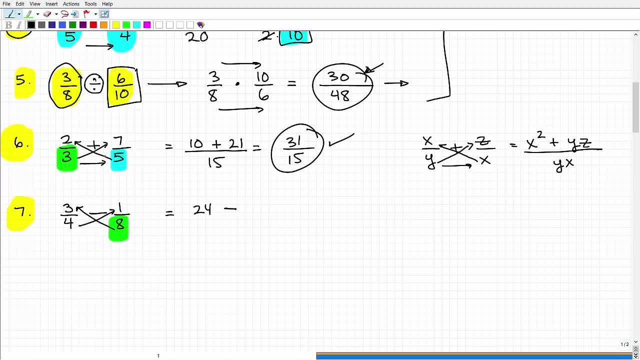 So that's going to be four times one. We're doing the exact same steps as the previous. problem is: uh, four over. That's our numerator of four times eight, which is what Thirty two. So our answer is going to be twenty over thirty two. 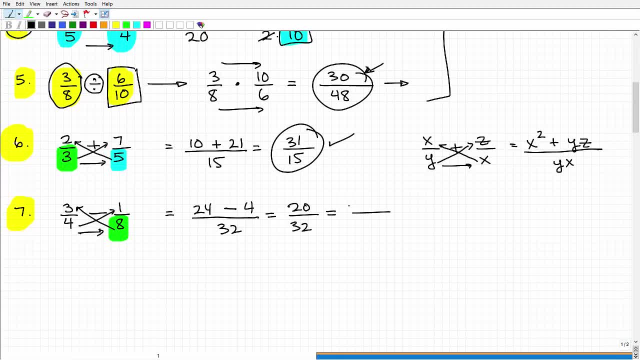 And, of course, we can reduce this: 20 is the same thing as 4 times 5, and 32 is the same thing as 4 times 8.. So I have these common factors which I can cross-cancel, and I'm left with my final answer. 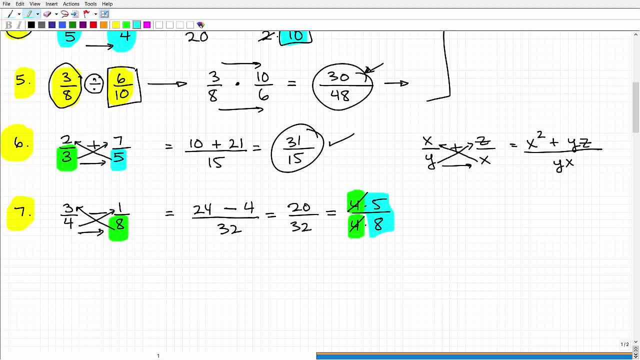 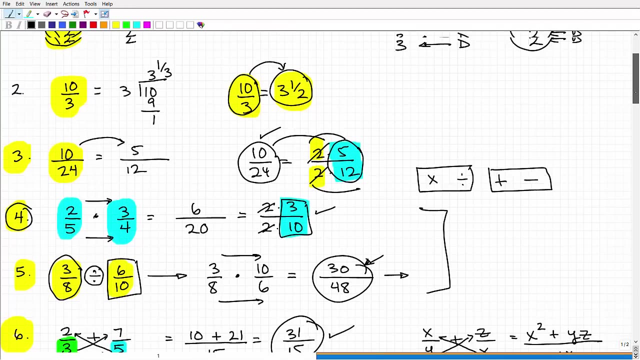 Whoops, I don't want that. I'm left with my final answer: 5 eighths, And that is it. So really, fractions. I'm not sure how long this video has gone, but you pretty much learned a month's worth of fractions, crash course. 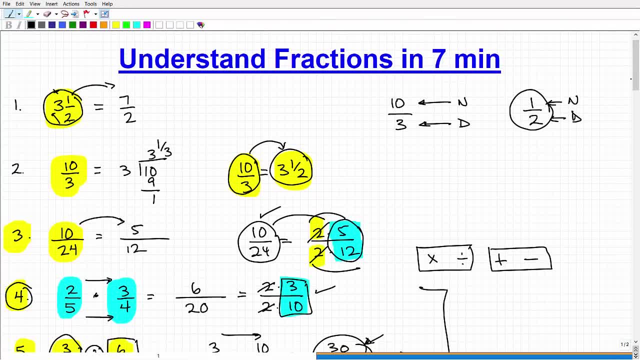 Hopefully. I'm sure I'm over 7 minutes, but who cares? The deal is that you know what. you probably remember all the stuff that you had to go through. Now there is obviously a few other things that you need to know with fractions.